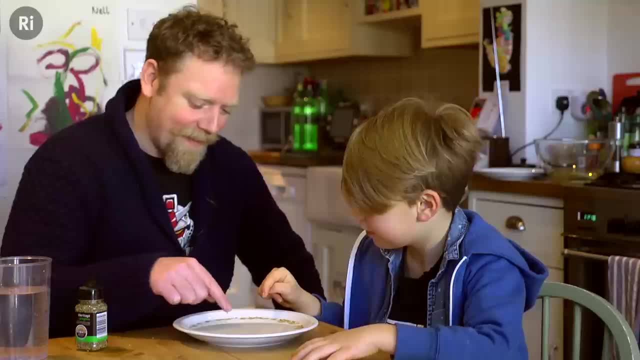 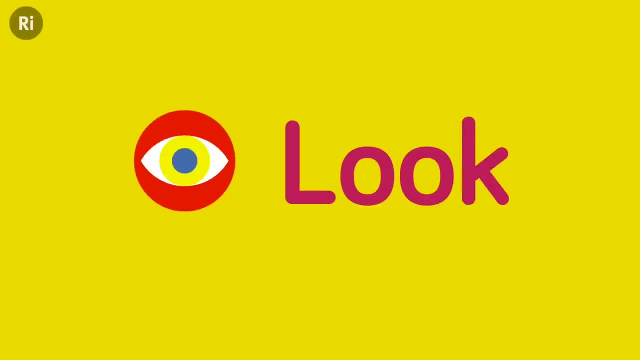 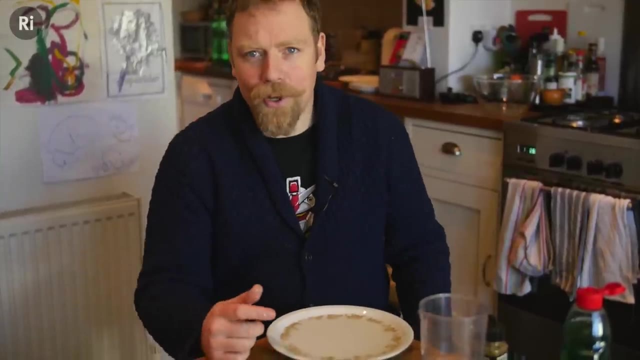 Wait, what is that green? What's that green? That is the washing up liquid that I secretly had on the plate. What's that green? That's the washing up liquid that I secretly had on my finger. Now, why is that happening? Imagine if you would a balloon. You've got that very thin. 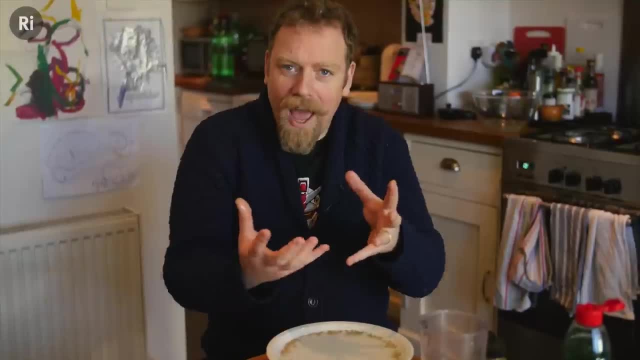 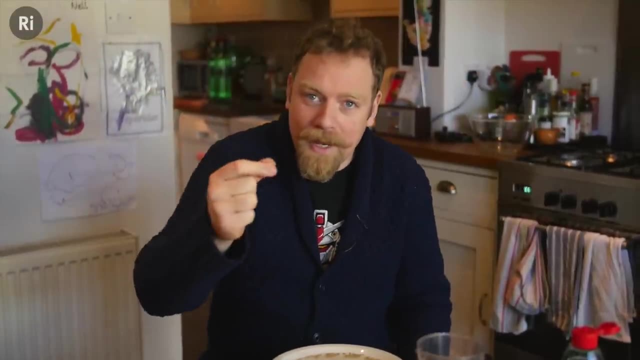 skin of rubber all around the outside of the balloon. You've got air all squeezed together on the inside of the balloon. It's basically pushing the skin of the balloon tight. Well, if you take a pin, then what you've done is you've weakened the skin of the balloon. 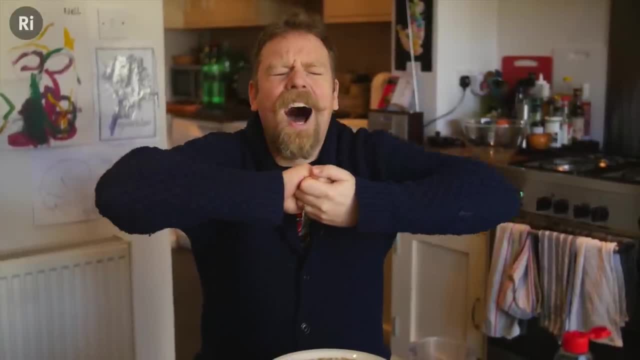 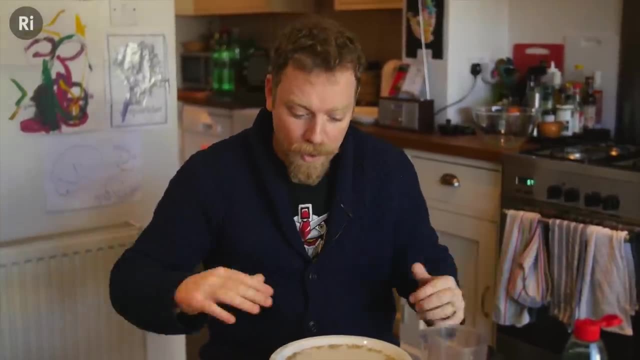 Essentially, all of those rubbery molecules that make up the balloon are going to be weakened. They're going to make up the balloon, They're holding onto each other really tight, and then you give it one little tear and the whole thing rips apart. 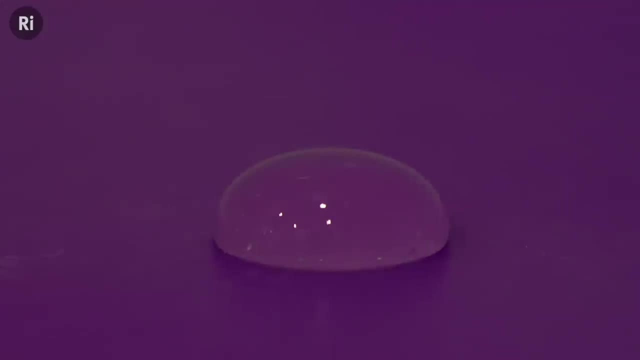 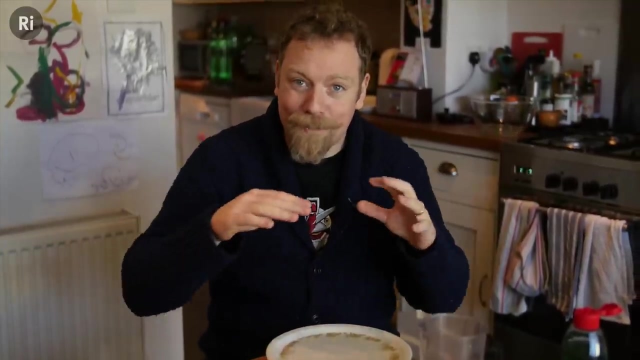 The surface of our water has this thing: surface tension. When we have that surface tension all those water molecules are holding onto each other really tightly. but what washing up liquid does is it breaks that surface tension. So if you break the surface tension in the 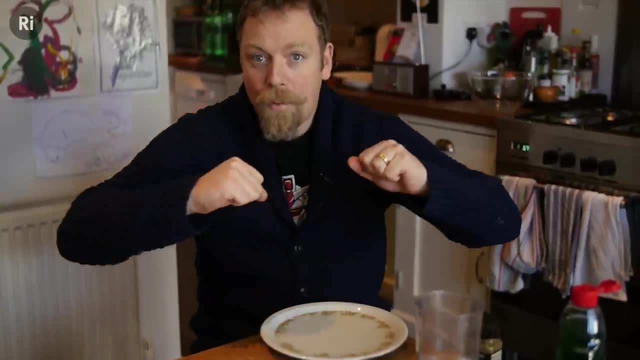 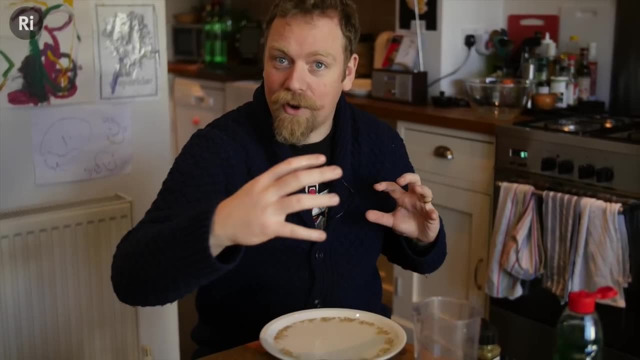 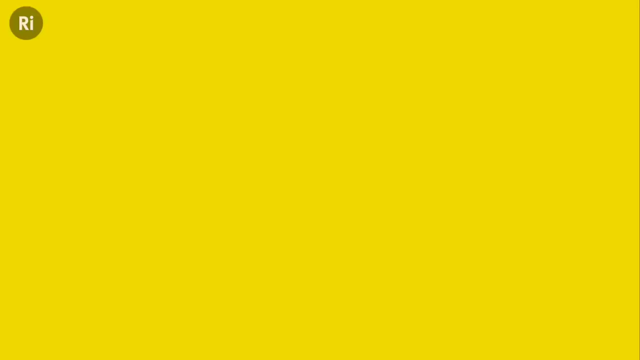 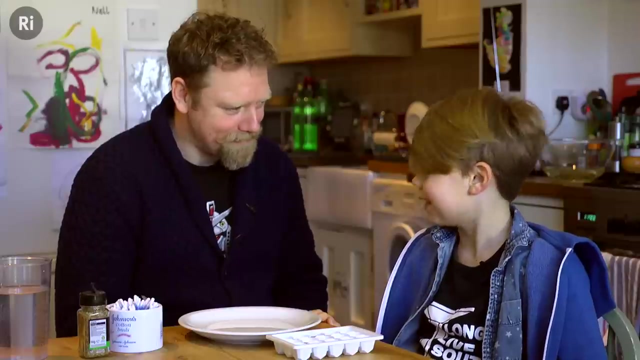 middle of that water. the other molecules all pull away from where the surface tension is broken, And when they pull away they drag the oregano with it. Can we use that important scientific discovery to have fun? Yes, we can, Albie. I thought we could try it with a few different things and see which one is the 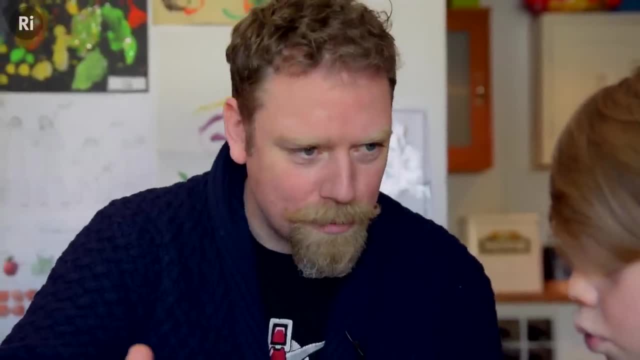 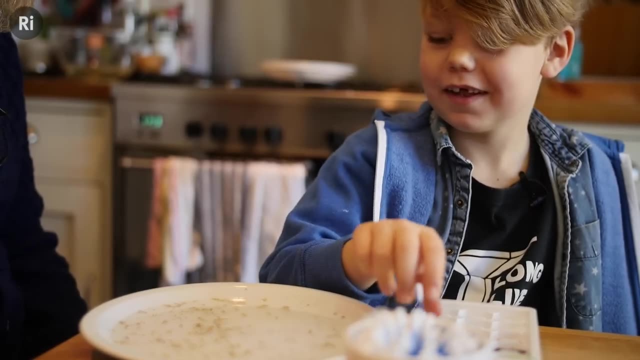 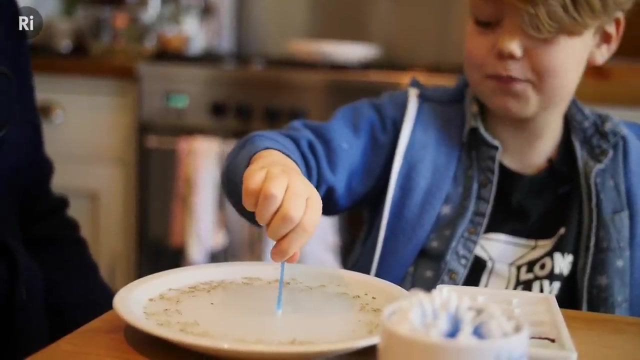 best. Okay, So we've got 10 things here in a little ice cube tray. What one would you like to try first? Hand sanitizer: What do you think might happen? I think the blood should go to the side again. The molecules will pull the oregano out to the side. You're right. 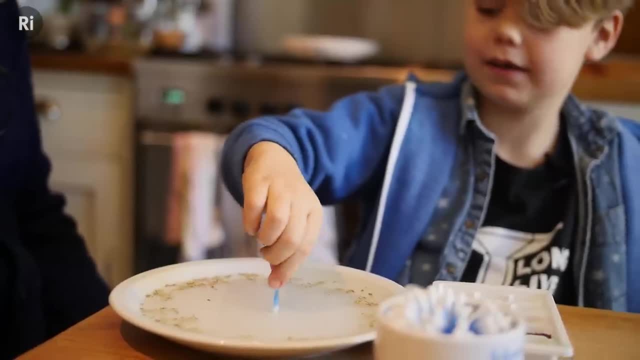 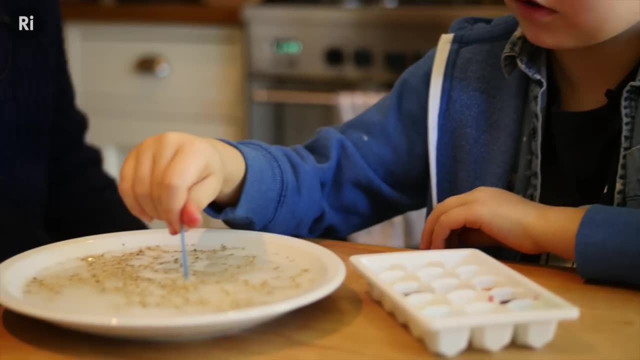 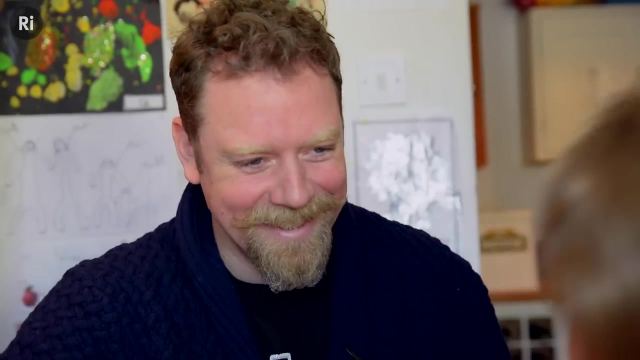 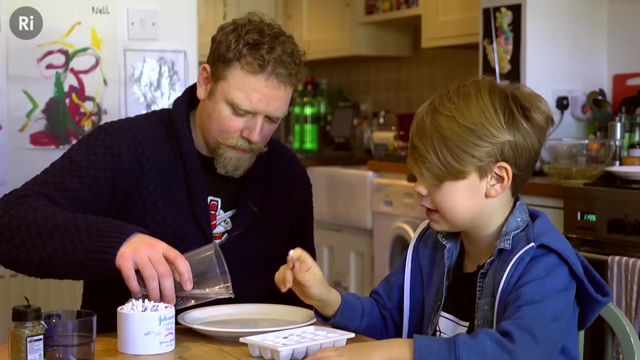 It's not the best, because last time it was like bright squished Okay. so why don't we write this down Now? the truth is, it doesn't matter if you understand all the real highbrow science to this, but it doesn't really matter if you can explain it to your kids either. The important 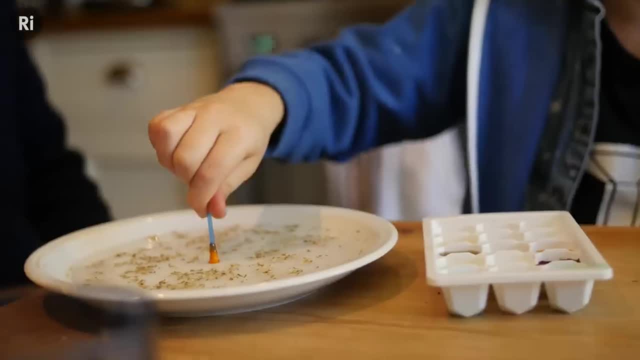 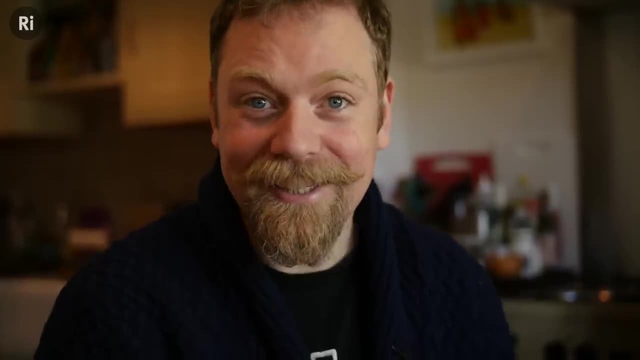 thing about this is that what we're going to be doing is testing, Taking an idea, trying lots of different versions of it, seeing what works best. That, my friends, is the scientific method. It's the underpinning of everything that's bought us: shoes, cars, penicillin. 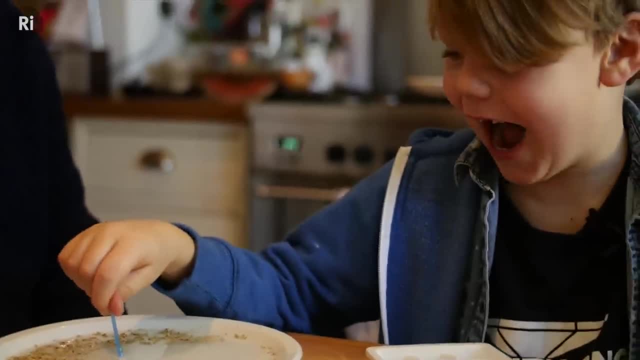 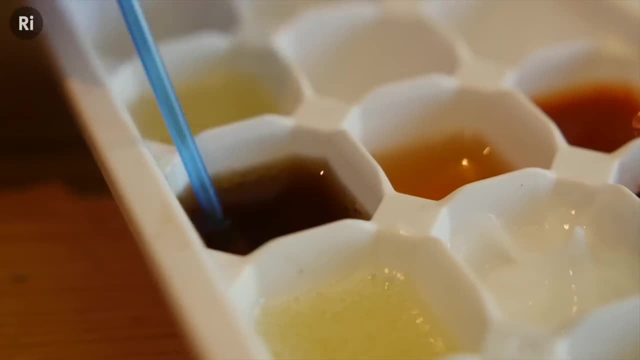 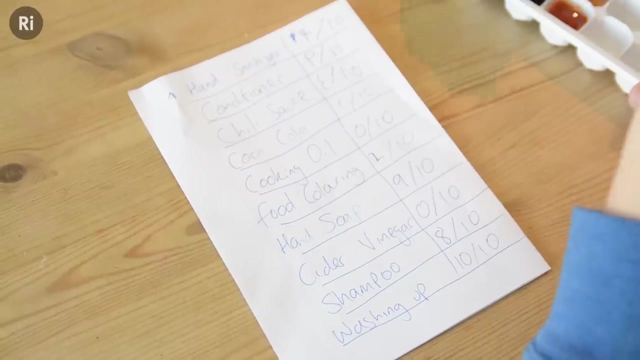 water. It's about having a way of thinking about the world that allows you not to be taken for a ride And, frankly, what better thing is there to give your kids than that? Wow, So what thing is best at breaking surface tension? 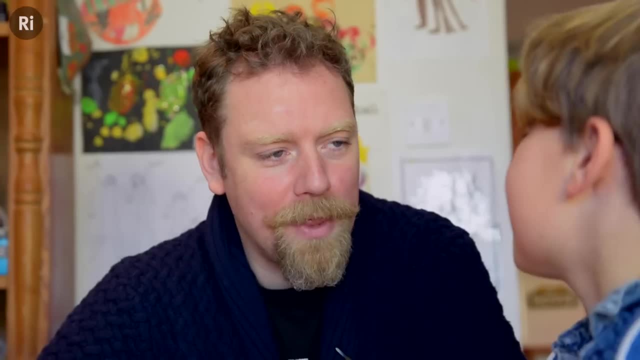 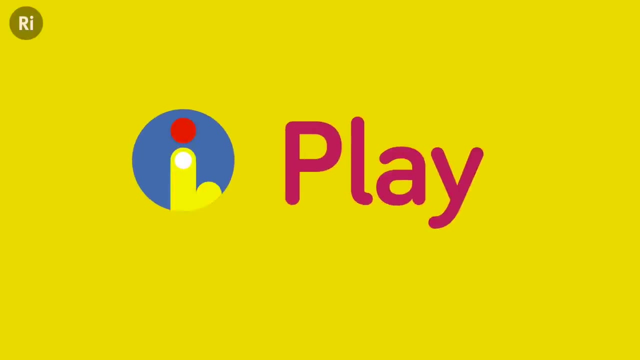 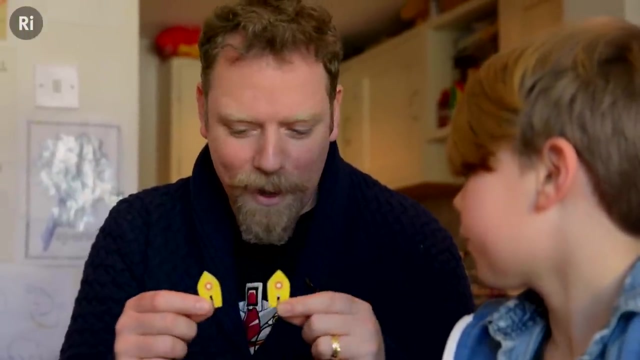 Washing up liquid, Definite, Definite. Shall we put that to the test? Let's put that one first. Okay, So out. What I've done is I've gone to the ORI website and I've downloaded templates to make these little boats All right. 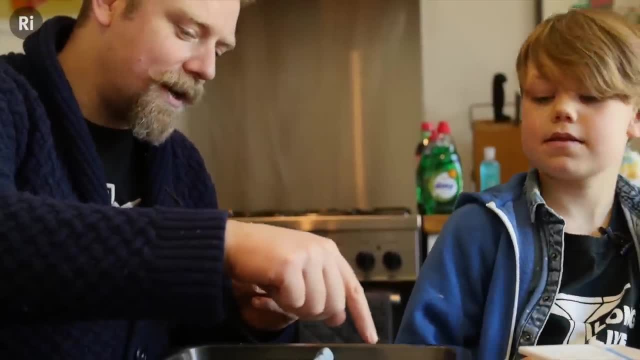 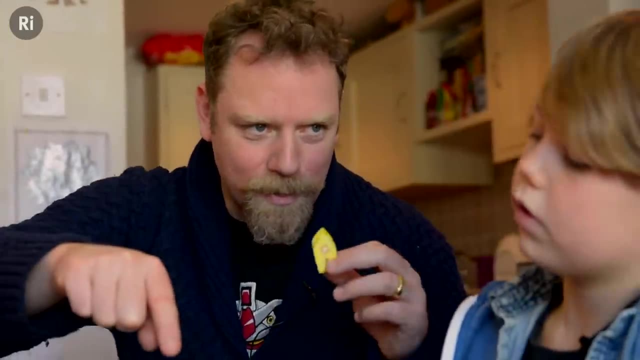 Right. So what we're going to do is you're going to have a boat on this side and I'm going to have a boat on that side. We're going to take some of this stuff that we've already experimented with and use it as our fuel. 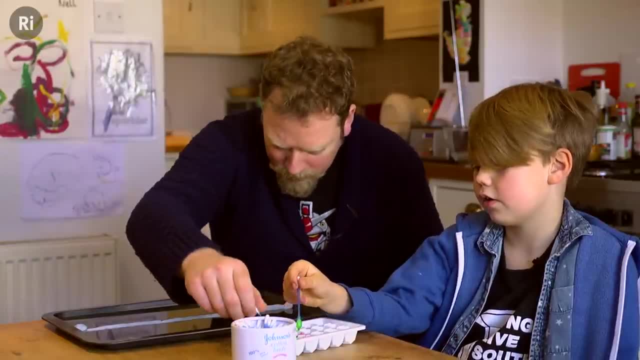 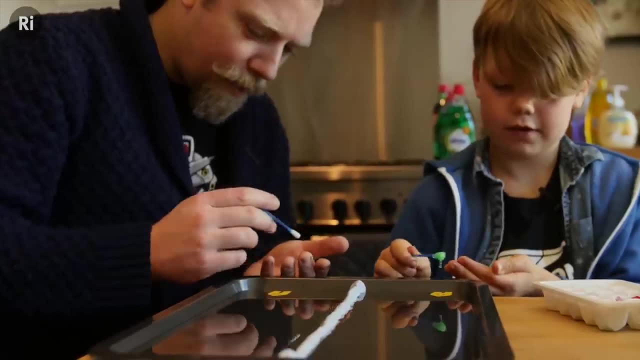 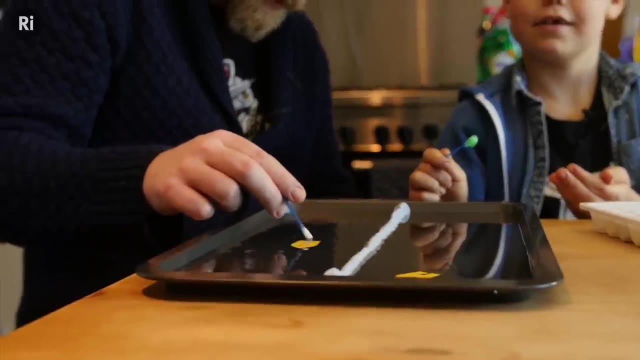 I show: All right, Ready, Yeah. So I'm washing up liquid. I'm going to use hand soap, which you scored nine out of ten. One, two, three, go. Yeah, Yours absolutely cruised up that end. Look, I'm going to have to have mine along. 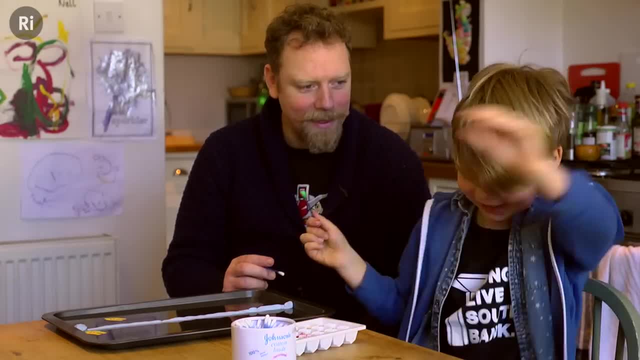 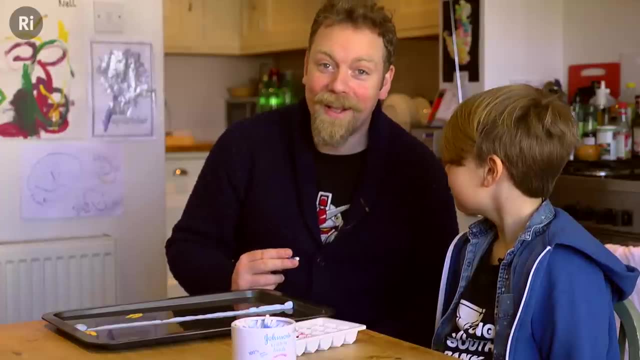 So washing up liquid was the winner, Yes. Albie was the winner, Yes, But Albie, Yeah- Was science the real winner? Yeah, Oh nice. If you'd like to try this experiment in your house with your own actual child, then you. 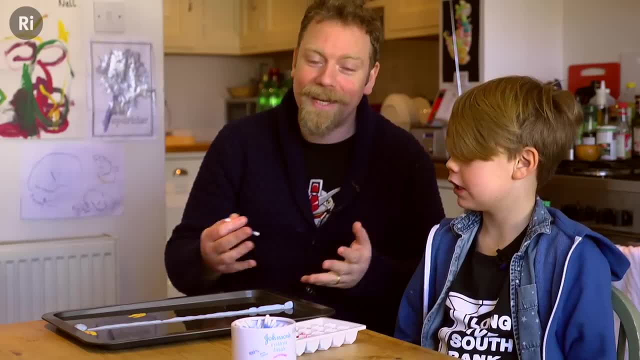 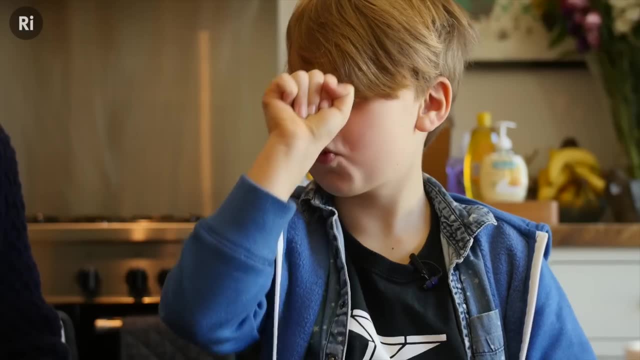 should. Why not go to the RRI website? All of the bits and pieces? you'll need some of the science explanation. that's all there. Alternatively, Albs people could subscribe to this channel and they would get new mind blown, right Mind blown.